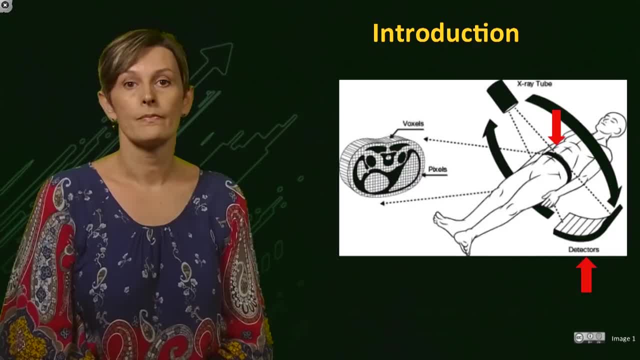 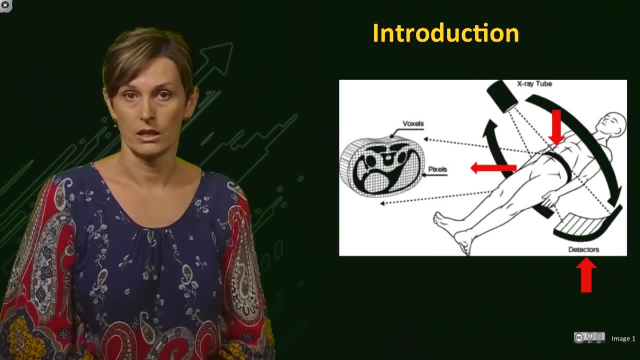 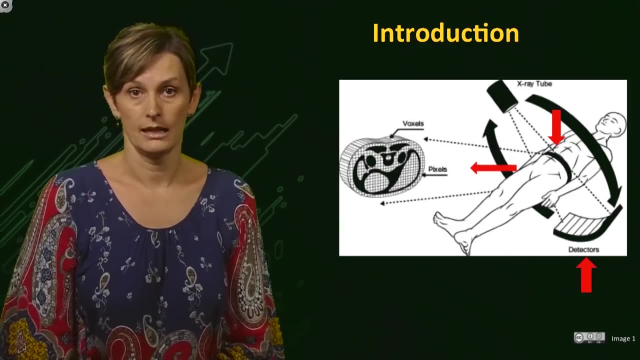 the same amount of X-ray radiation passing through the different organs and getting unto electrical signals. Those signals are processed by your computer, using different algorithms, to create CT images. If we use a simple X-ray system, only a two dimensional image can be created. However, with CT technology, by measuring radiation going through the 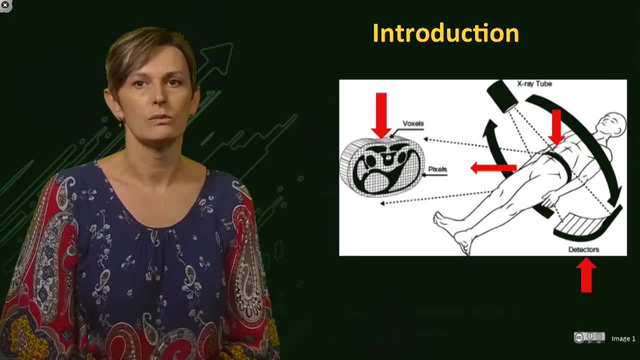 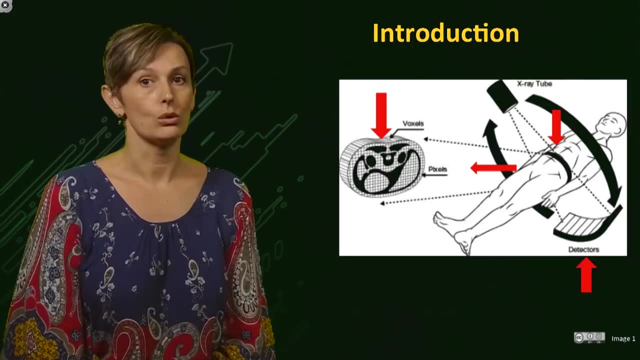 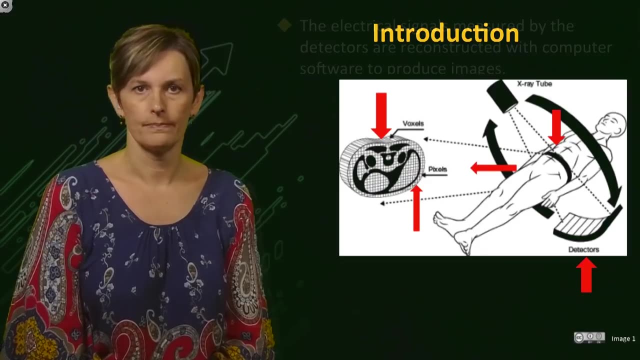 body at different angles, we can now make three dimensional pictures. The computer here plays a key role, splitting up organs in the body into small volumes called voxels. A voxel is a three-dimensional equivalent of a pixel. Now that the data have been acquired, the next step is to produce the images. 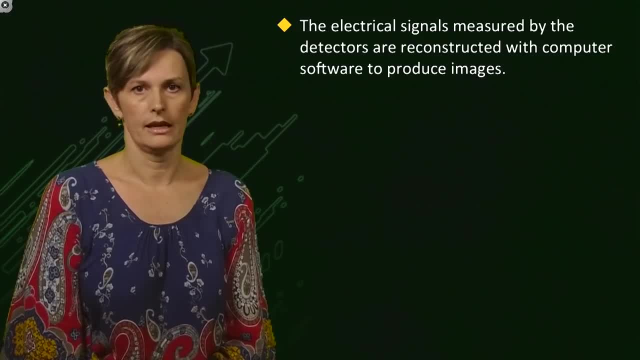 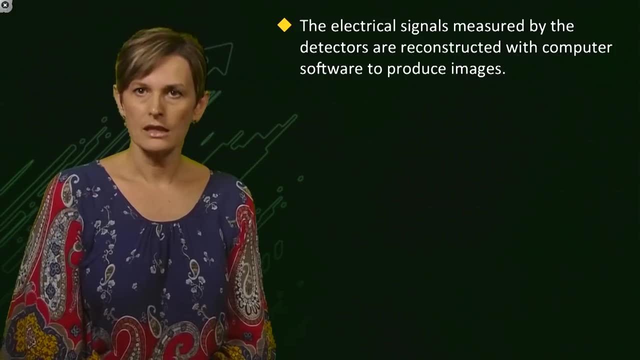 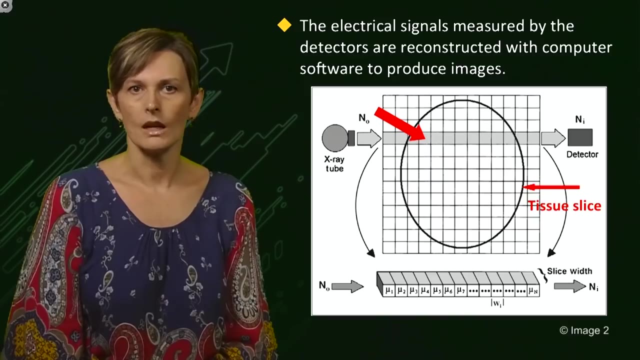 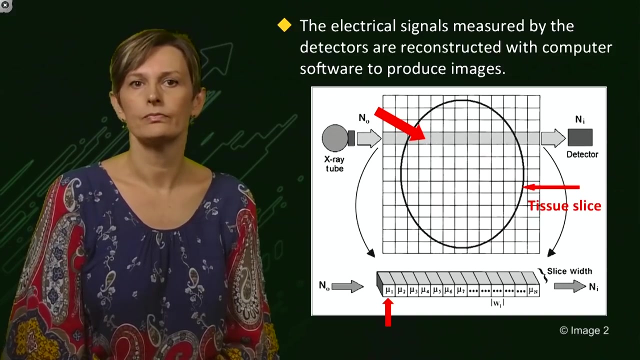 The electrical signals measured by the detectors are reassembled together with a computer software creating images. For example, in this figure, each voxel from a scanned body part is allocated a number, also called an attenuation coefficient number, mu. The mu value represents the level of attenuation of the X-ray going through the body parts. 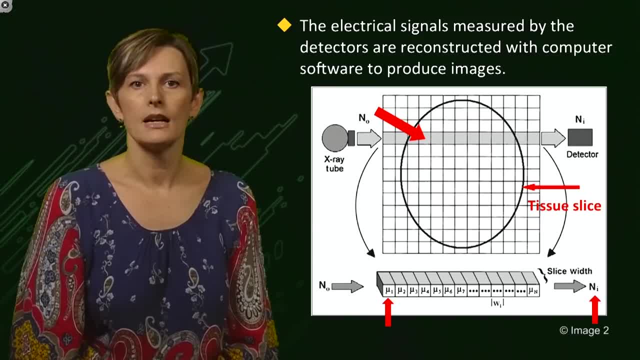 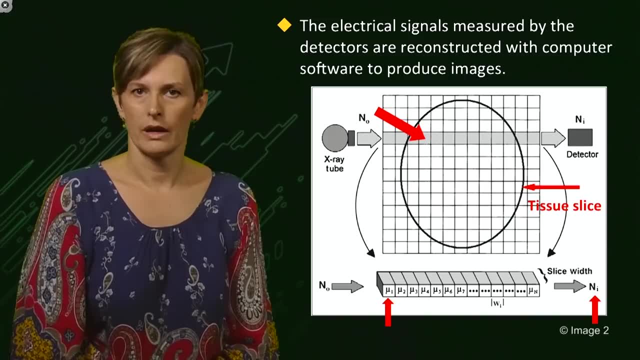 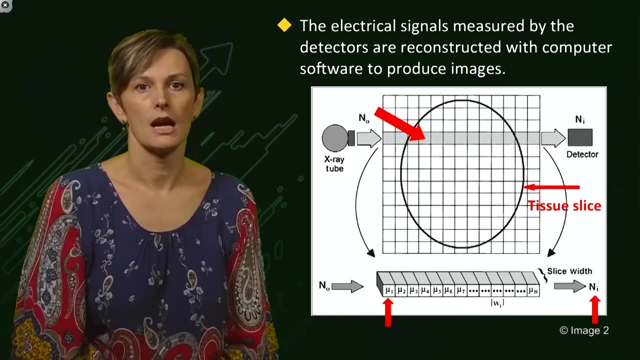 The X-ray transmission measurement, Ni, represents the sum of all attenuation values from all voxels in each distribution. For example, the voxel from bone will have high mu value due to very high attenuation of X-ray radiation, But the voxel from skin will have low mu value as the skin has very low X-ray attenuation. 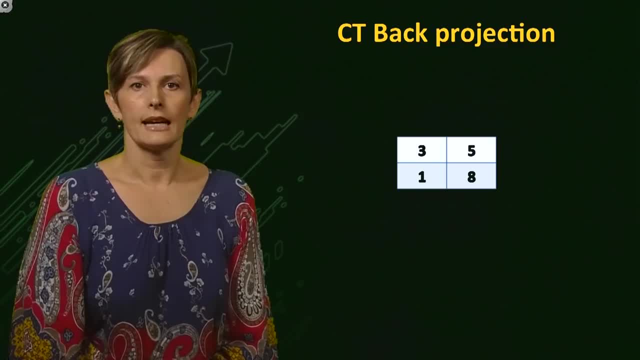 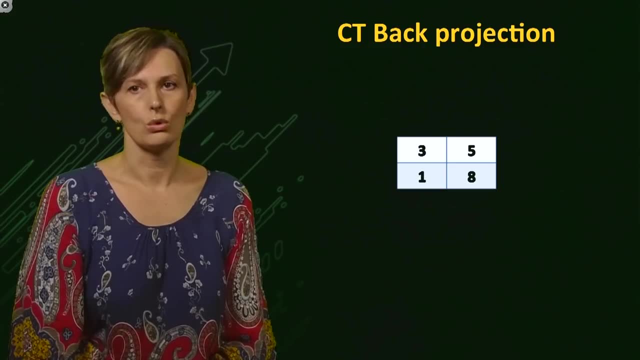 Let's take an example of a voxel from a tissue slice. I have assembled them in two rows and two columns. I have also assigned some random attenuation values to the voxels. I have assigned a value of 3,, 5,, 1 and 8 to each voxel. 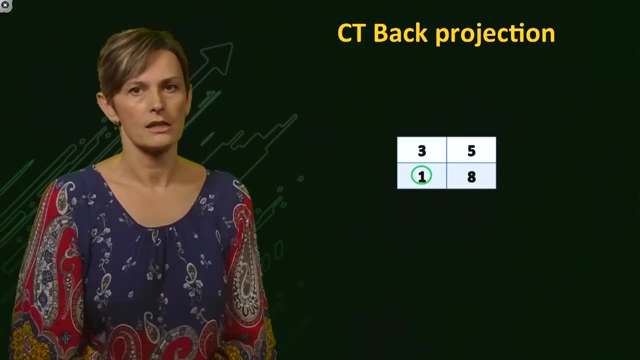 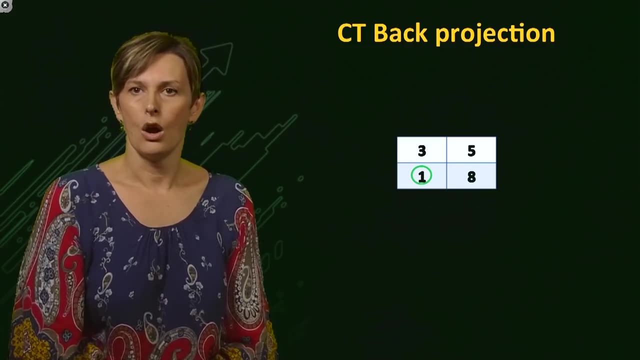 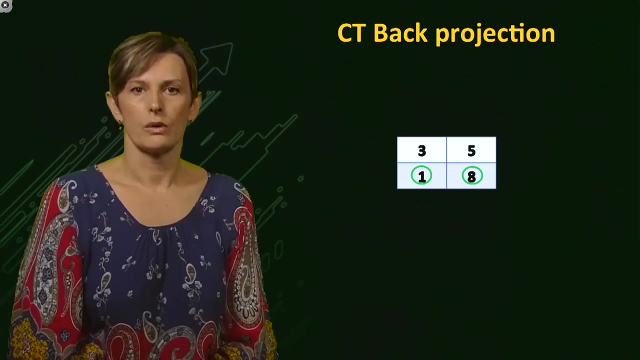 In this case a value of 1 will represent no reduction of radiation intensity, meaning a low attenuation of X-ray by the tissue. A value of 8 will represent here a maximum attenuation of the X-ray. The X-ray passes through the tissue slice at different angles. 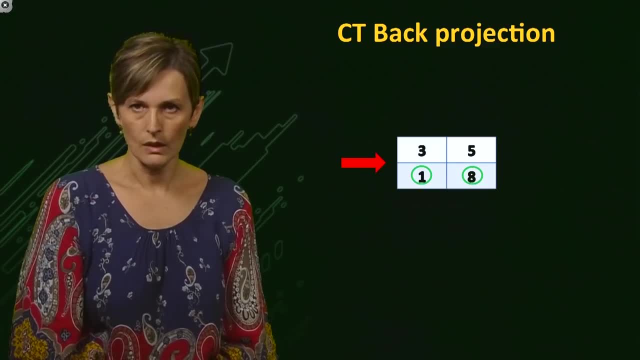 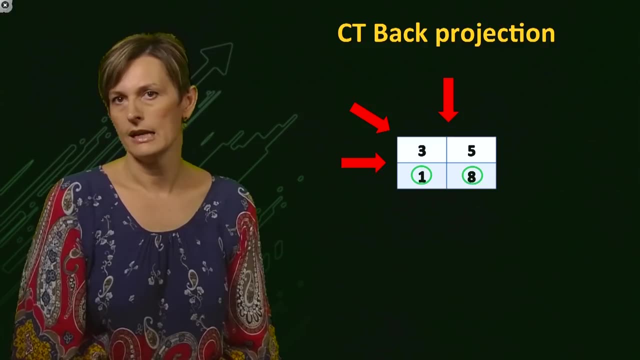 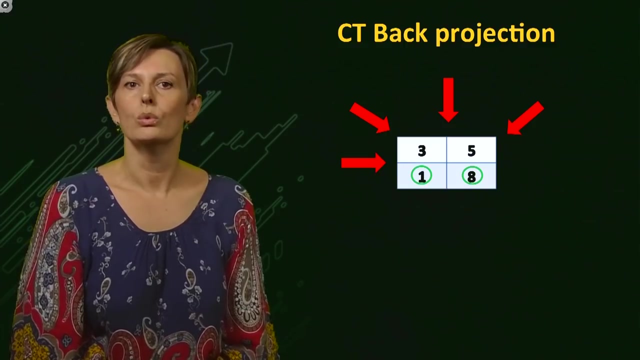 0 degrees will come from left to right, 45 degrees angles diagonal, Then 90 degrees from the top to the bottom And finally, 135 degrees angle will be diagonal. on the other side, Each attenuation value will be expressed as a sum of the voxel attenuation value along the radiation path. 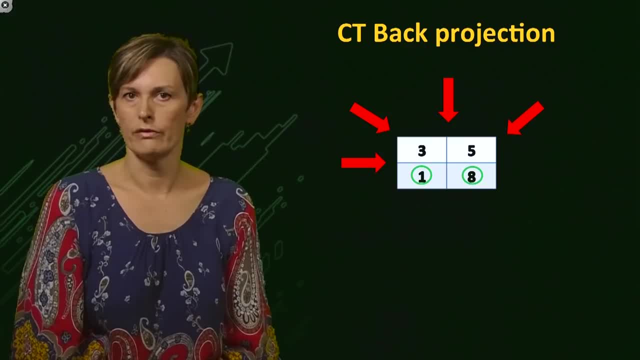 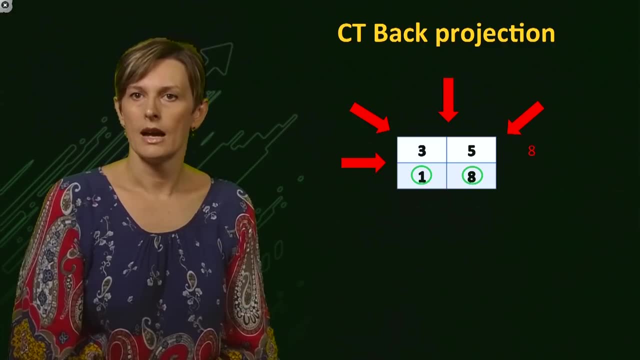 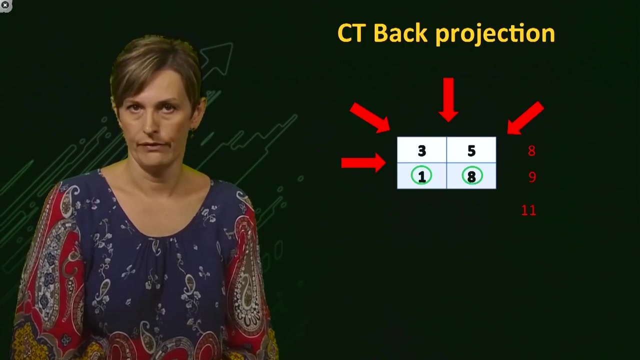 So in this example, the new attenuation value after X-ray radiation from the 0 degree angle will be then 8 and 9.. From 45 degrees the new value will be 11. And then from the top, at 90 degrees, the value will change to 4 and 13.. 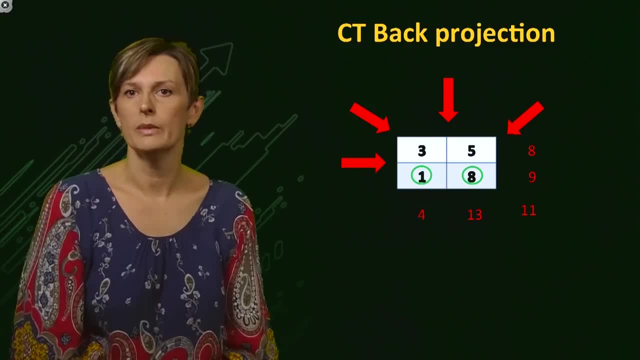 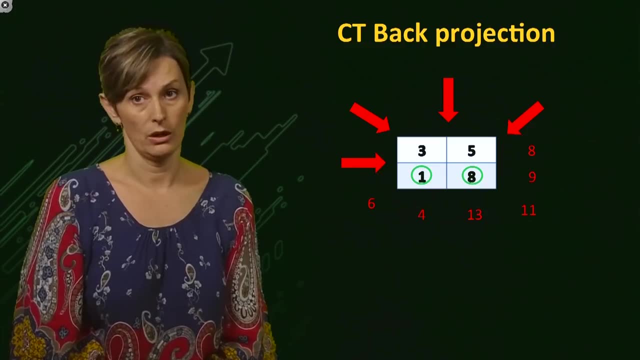 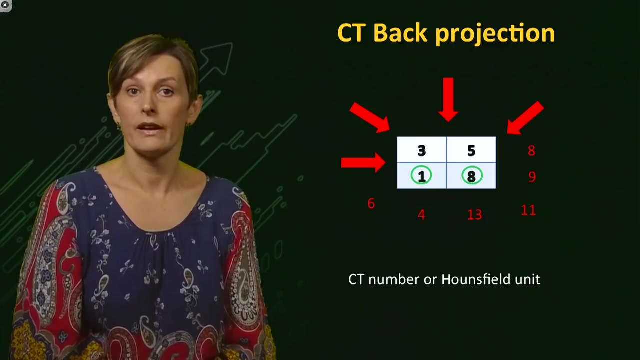 And finally, at 135 degrees, the new value will be 6.. An agreement from the earliest days of CT is to replace the name attenuation value by CT numbers or Anfield units. The Anfield unit is a concept that we actually will discuss a bit more during this course. 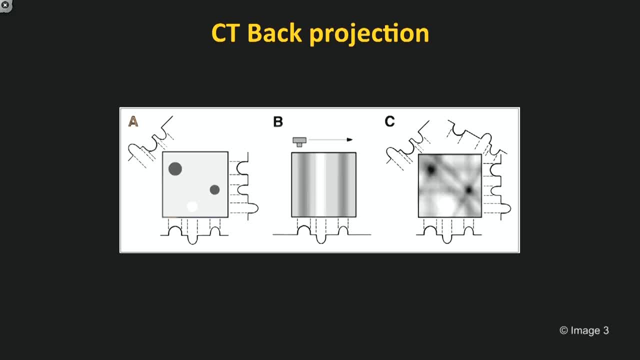 To understand back-projection reconstruction, let's try with another example here showing a CT scan of an object. This object has three different attenuation materials. The attenuation values from each view taken at different angles are divided evenly along the path of the ray showing here. 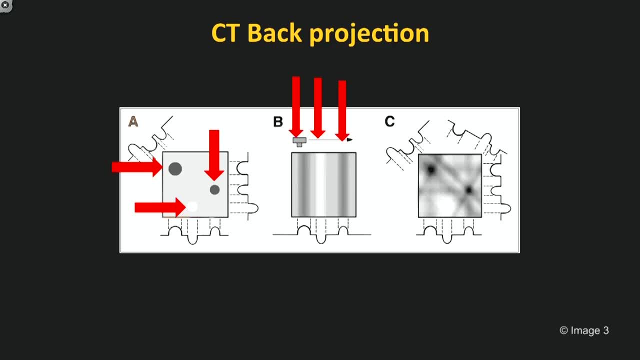 This process is called back-projection. In the figure C, as you can see, after back-projection the four views are summed together, And here it's a different direction And an image of the test object is beginning to appear. It is quite blurry at first. 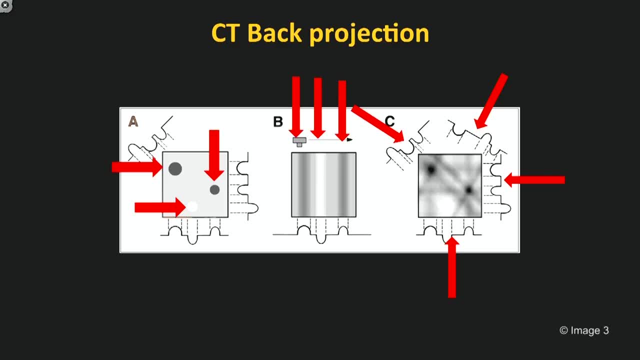 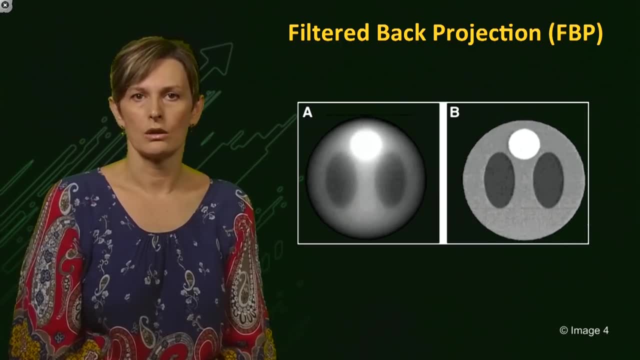 but the quality of the image can be improved by using a mathematic process Such as filtering. To understand the importance of filtering, let's compare two pictures. The first picture is a CT scan image of an object before mathematical filtering, And here is the same picture after filtering. 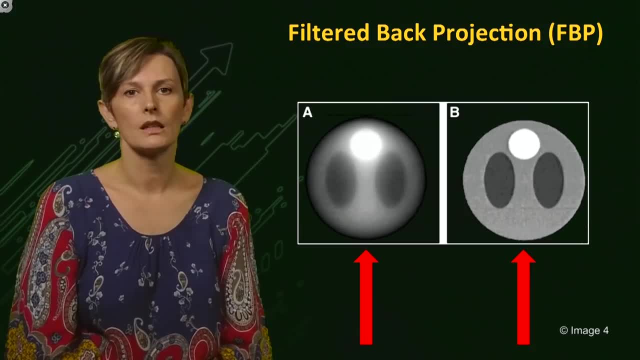 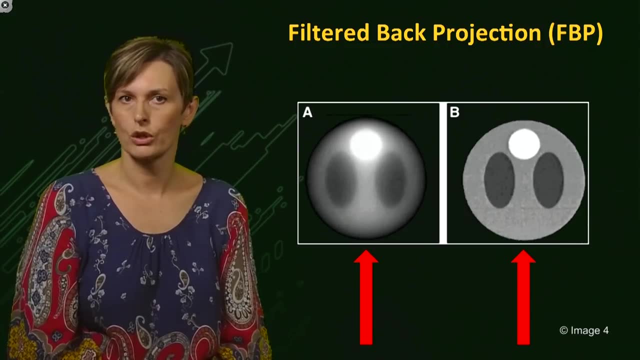 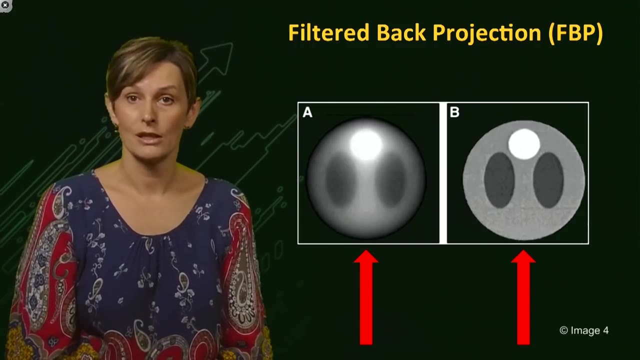 As you can see, the image becomes much sharper. To summarize, in this section we have covered some of the basic principles of image reconstruction and filtered back-projection for computed tomography. If you want to learn more about these topics, you can view Dr Andrew Jahnke's presentation. in the Advanced Topics section. 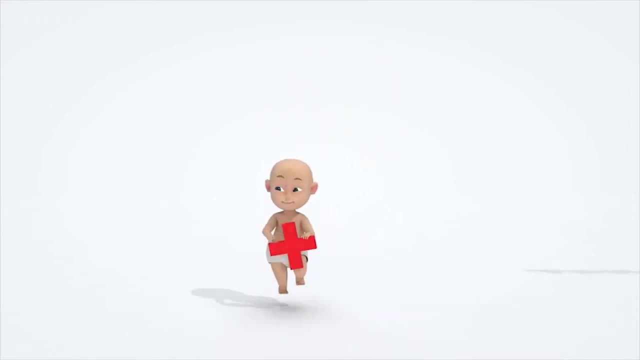 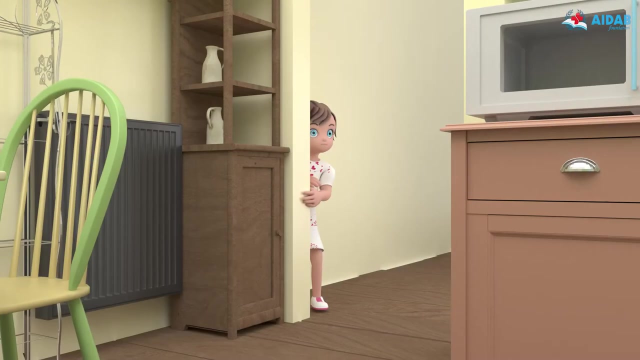 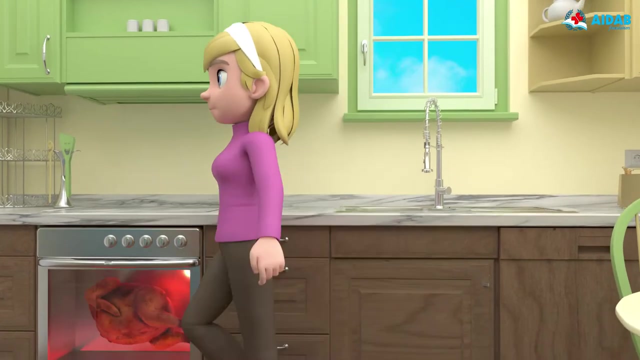 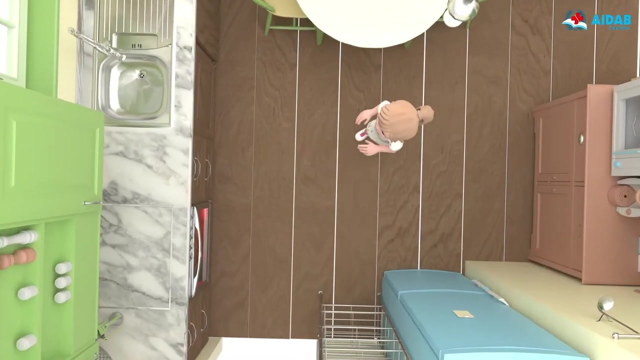 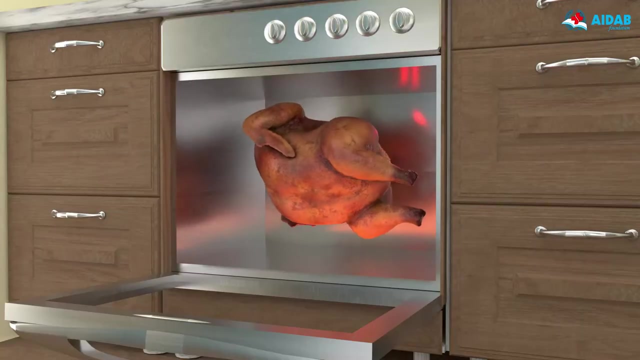 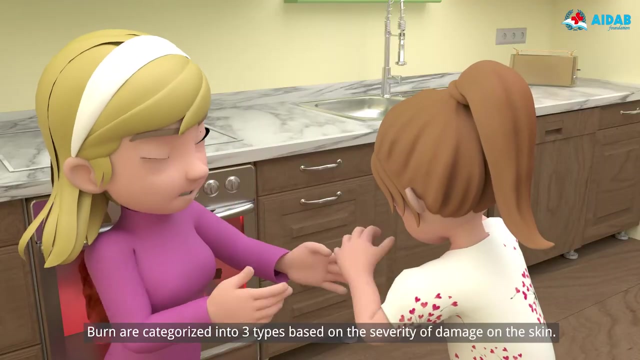 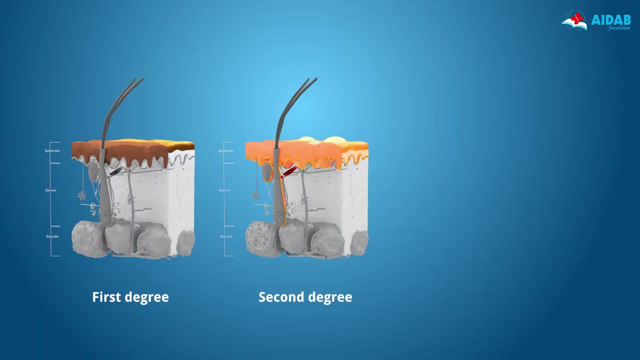 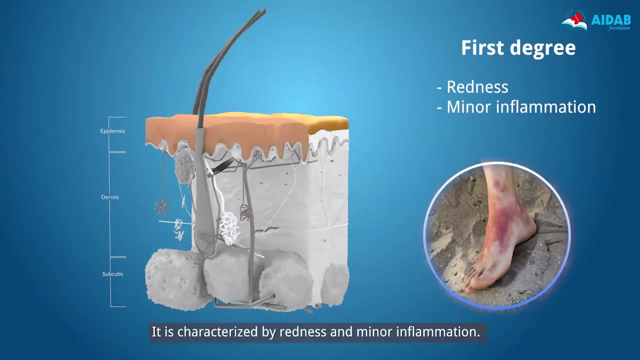 good luck. Burn are categorized into three types based on the severity of damage on the skin: First degree, second degree and third degree. First degree burn only affect the top layer of the skin. It is characterized by redness and inflammation. 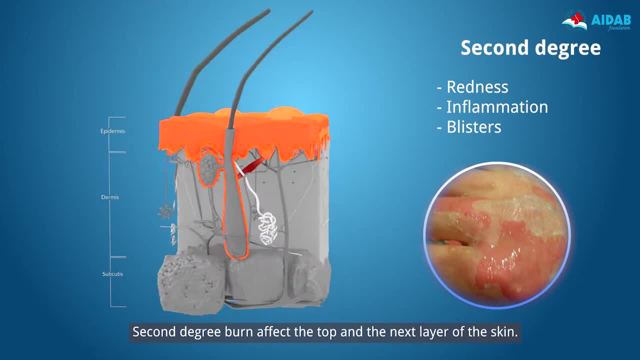 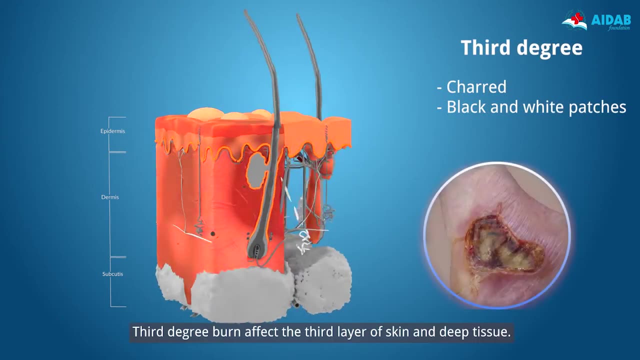 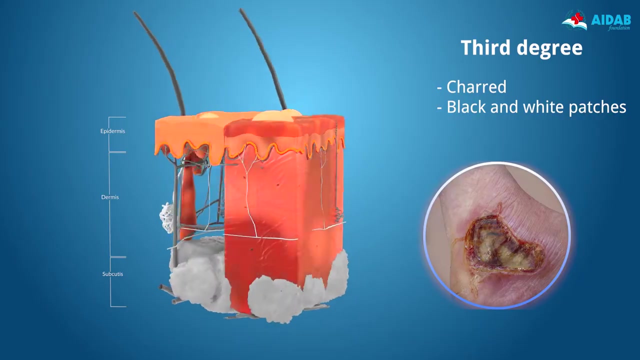 Third degree burn affect the top and the next layer of the skin. It is characterized by redness, inflammation and blisters. Third degree burn affect the third layer of skin and deep tissue. It is characterized by charred, black and white patches. 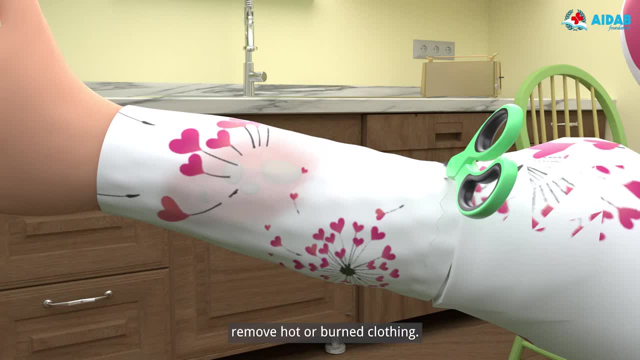 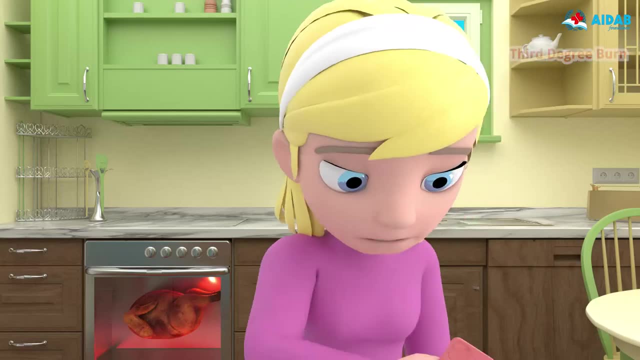 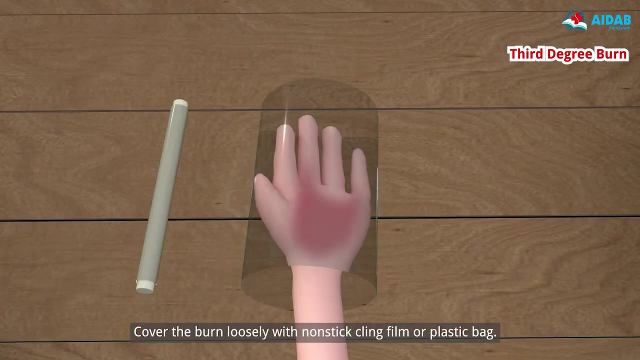 For all burns. remove smoldering materials. remove hot or burnt clothing. If clothing sticks to skin, cut or tear around it For third degree burn. call a local emergency number immediately. Cover the burn loosely with non-stick cling film or plastic bag. 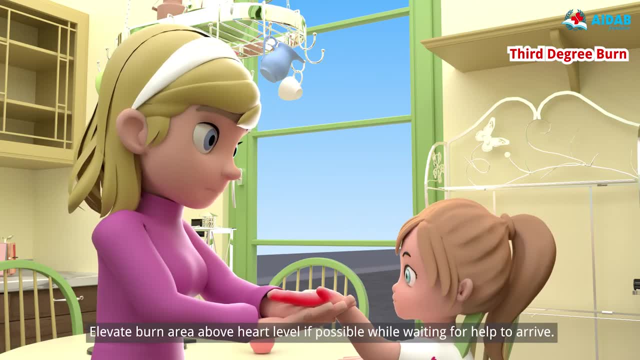 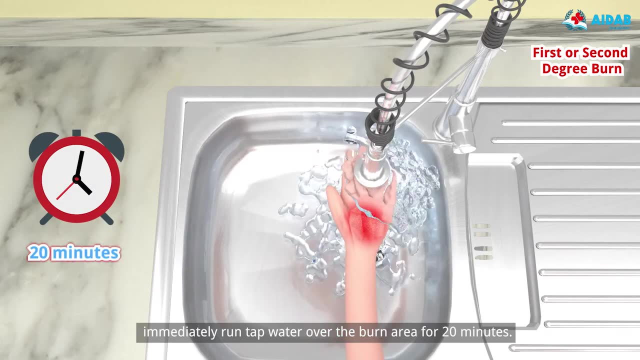 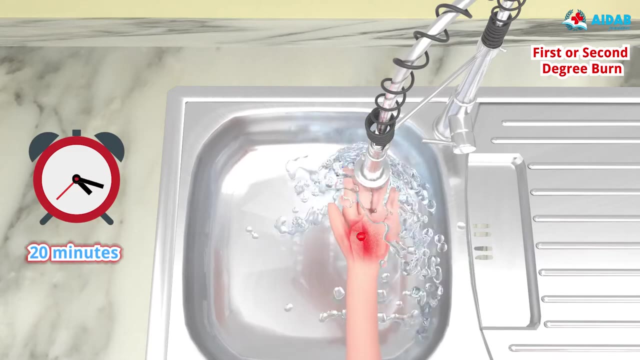 Elevate burn area higher than heart level if possible. while waiting for help to arrive For first and second degree burn, immediately run tap water over the burn area for 20 minutes. This will help to reduce swelling, pain and chance of scars. 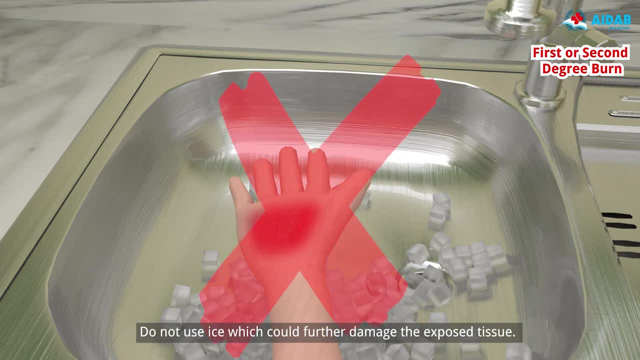 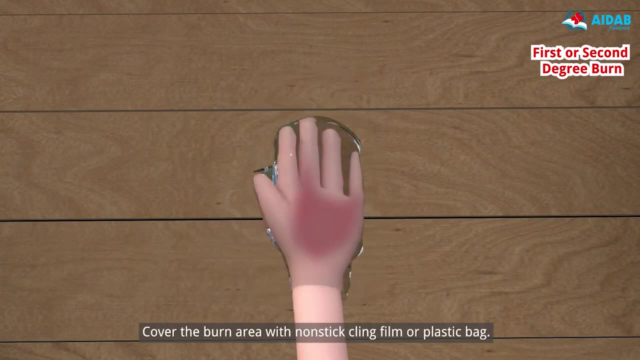 Do not use ice. It is recommended to use a non-stick cling film or plastic bag, which could further damage the exposed tissue. Do not break blisters. Cover the burn area with non-stick cling film or plastic bag. If sign of infection-like smell has developed, see your doctor immediately.